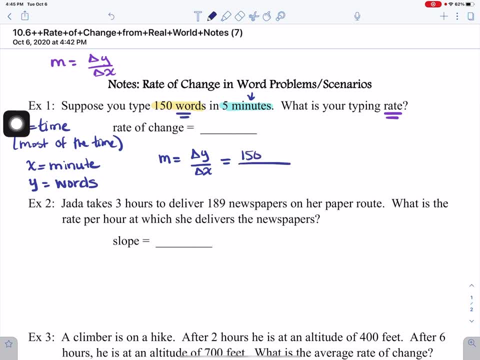 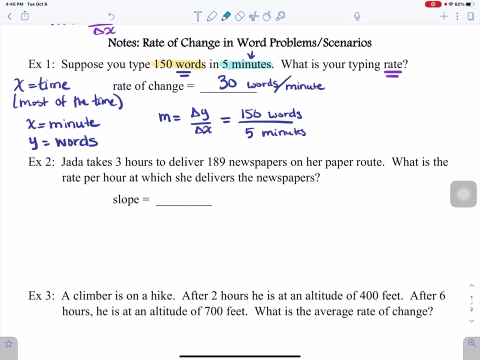 words. We'll put 150 words And then time will be our x value, which is five minutes. So 150 divided by five is 30 words per minute. Our next problem We have: jada takes three hours to deliver 180 words to Jada We're going to have to divide 150 words by five. 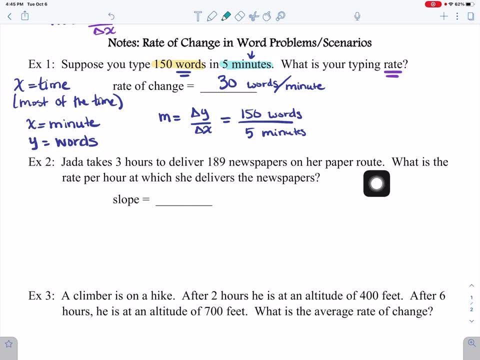 And then we're going to put 150 words in five minutes. So that's half the change and That's half the change. So that's half the change. newspapers on her paper route. What is the rate of per hour at which she? 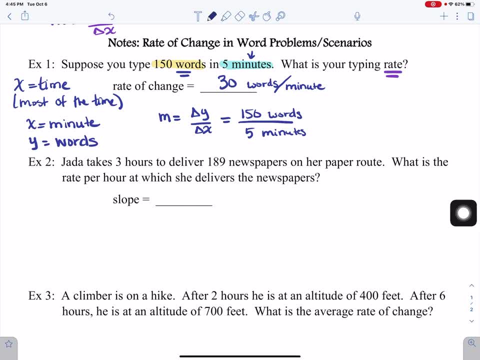 delivers the newspaper. So they're asking the rate per hour. So we're doing rate of change. What's important about it? we have three hours. Excuse me, meant to highlight that Three hours. she delivers 189 newspapers. Now we have hours in newspapers Now at number one I mentioned. 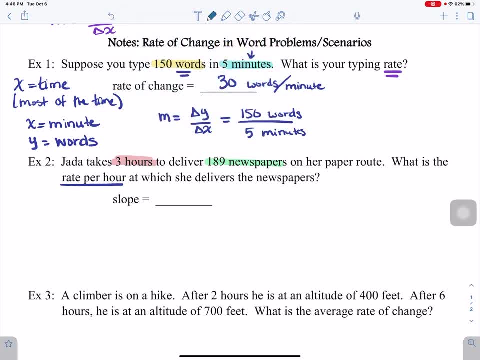 that time is X, So our time will be hours and Y will be hours. So our time will be hours and Y will be hours. So our time will be hours And Y will be hours. So our time is hours And Y will be hours. So our time will be. 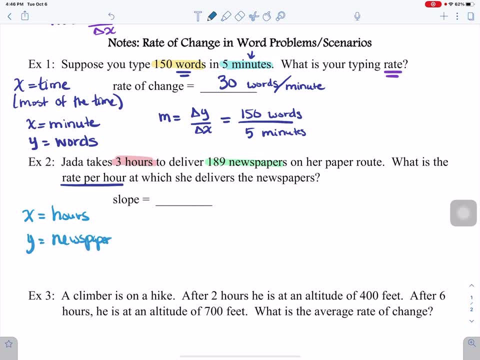 are newspapers, so it's 189 newspapers. that goes on top because remember the change of Y over the change of X divided by our time, which is 3 hours. so 189 divided by 3 is 63 newspapers. excuse me, newspapers per hour. okay, so number one. 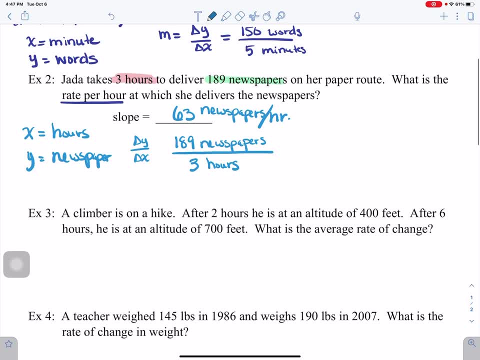 and two had two numbers. but look at number three. number three, even before we start, has one, two, three, four, four numbers. so let's go ahead and read it and see what they want. looking at the question, my keywords are ready to change. so this one says a climber is on a hike. after two hours he is at an altitude of 400 feet. 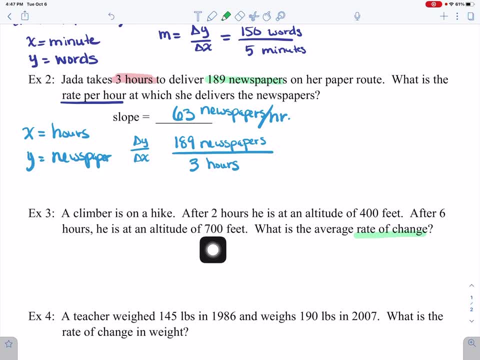 after six hours he is an altitude of 700 feet. what is the average rate of change? well, he is in two hours. he's in what altitude? 400 feet, and it says that in six hours he is in 700 feet. so here we have feet verses time. so I'm gonna go ahead and 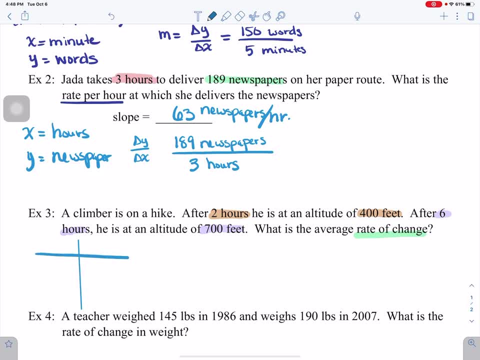 create a table. so I mentioned that time is X, so hours will be Rx And our altitude feet will be our y. So in 2 hours he is in 400 feet And in 6 hours he is in 700 feet. So what is the change of x from 2 to 6?? 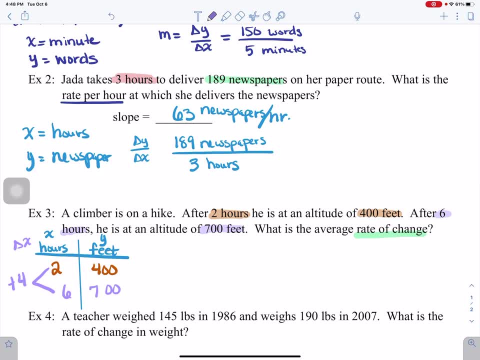 The change was positive plus 4 hours. And what is the change for y between 400 to 700?? Well, it changed by adding 300.. Remember to find the slope. you do the change of y over the change of x. 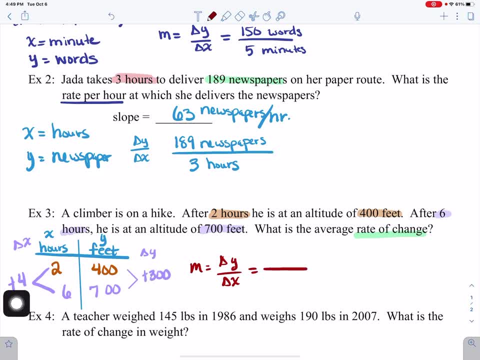 Or the way that it changed for y It was 300 feet And the way that it changed for x it was 4 hours. So 300 divided by 4 gives us 75 feet per hour. Okay, going to the next one. 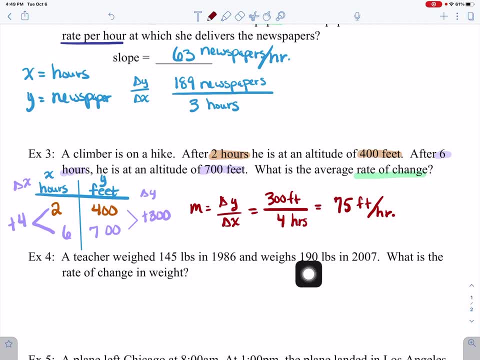 How many numbers do we see? 1,, 2,, 3, 4.. What are we finding? We're still finding the rate of change. Now let's read the problem: A teacher weighs 145 pounds in 1986 and weighs 190 pounds in 2007.. 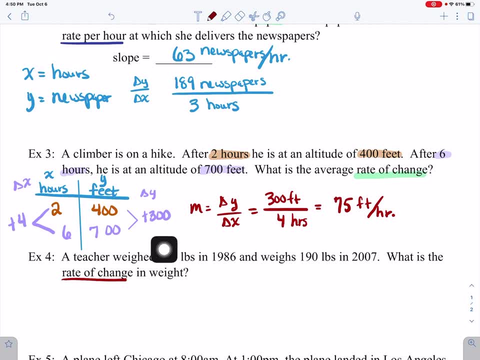 What is the rate of change in weight? Well, let's go ahead. We are going to create a table. I'm going to mark important information. So this teacher weighted 145 pounds in the year 1986 and 190 pounds in the year 2007.. 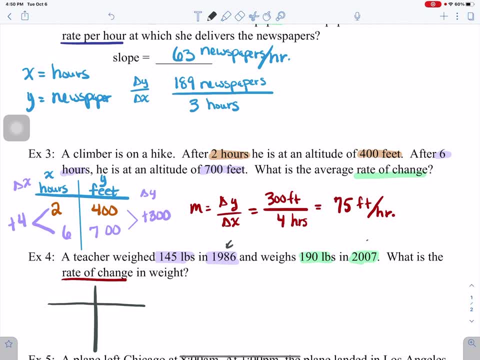 So again we have time which is in years, That will be in years. our X, So that means our weight, that is in measured in pounds, will be our Y value. So in 1986 the teacher weighted 145 pounds and the year 2007 the teacher 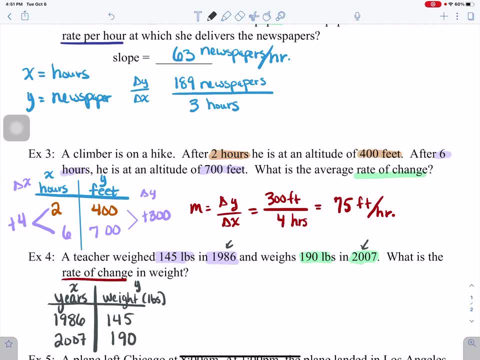 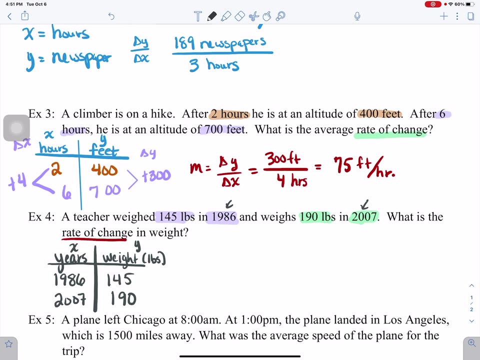 weighted 190 pounds. So now we have to find how it changes for X and how it changes for Y. Go ahead and pause the video and then see if you have the answer correct. So go ahead and pause it and then come back when you're done. 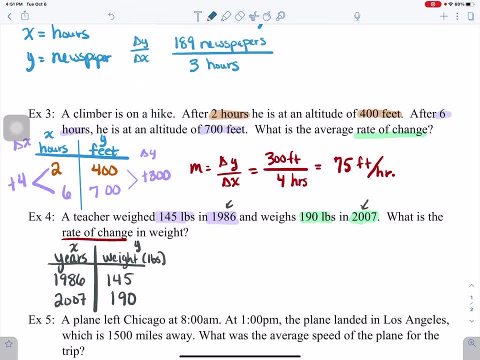 Okay, welcome back In the years, the way that it changed for X. So they added 21 years and the change of Y from 145 to 190, it was plus 45. So we did the change of Y over the change of X. 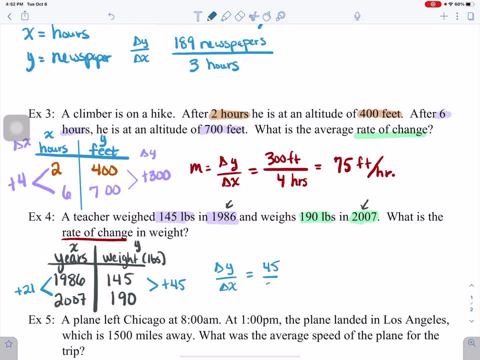 45 goes on top because that's the change of Y and 21 goes on bottom because it is the change of X. And we're talking about pounds and years. 45 divided by 21,. this teacher gained weight about 2.14, and we round it two places after the decimal 2.14 pounds per year. 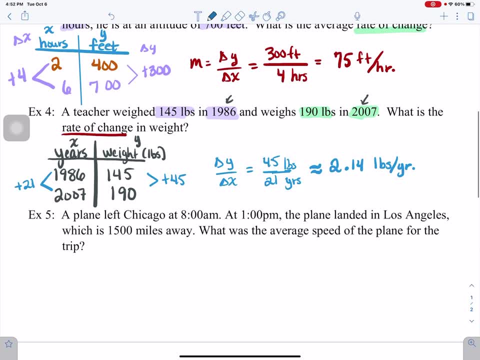 Okay, let's go to number five. Okay, before we start on number five, let's see how many numbers are given to us: At 8 am, At 8 am, 1 pm and at 1,500 miles. 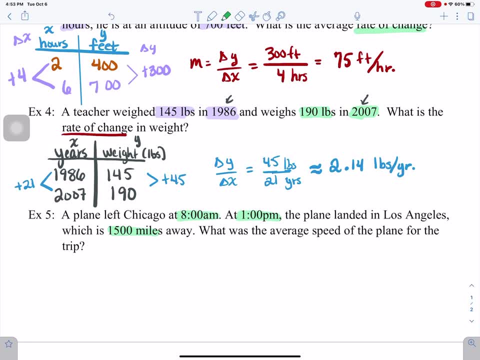 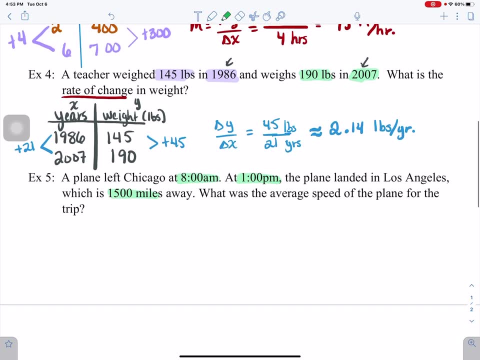 So this one only shows three numbers. Well, what happened to the fourth one? Well, let's go ahead and read it. It says: a plane left Chicago at 8 am and at 1 pm the plane landed in Los. Angeles. 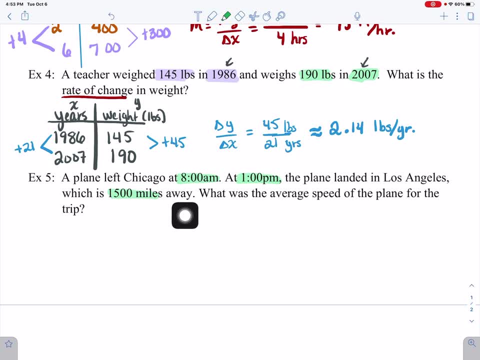 which is 1,500 miles away. What was the average speed of the plane for this trip? Well, let's go ahead. Go ahead and pause the video. See if you could go ahead and create your table. Go ahead and pause it and then come back. 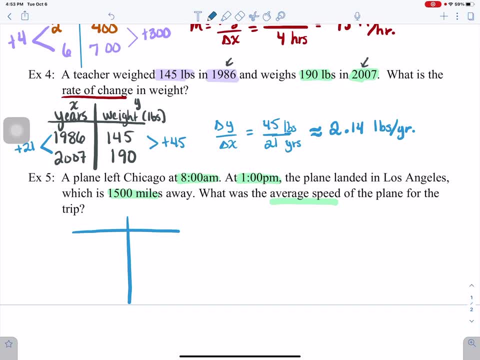 Okay, welcome back. Well, we're talking about 8 am and 1 pm, so that's time, That is time in hours. So that will be our x And then our y will be our miles. So this plane left at 8 am and it landed at 1 pm. 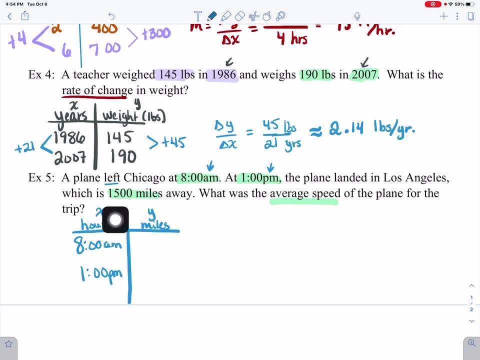 Okay, Now we have one more number. It says: at 1 pm the plane landed at Los Angeles, which is 1,500 feet away. Excuse me, So at 1 pm it landed from Chicago to Los Angeles at 1,500. 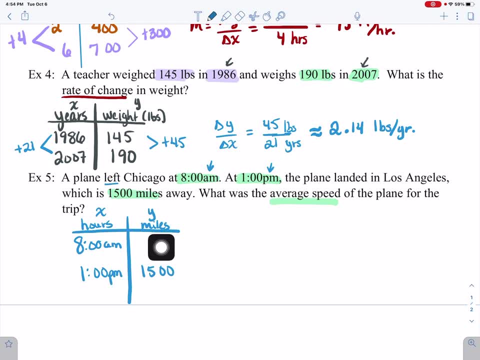 So what did y'all put here? Well, if it leaves at 8 am, it has. It cannot travel, so it starts at zero miles. So let's go ahead and see. Be careful here. This is here. We start at am, at 1 pm. 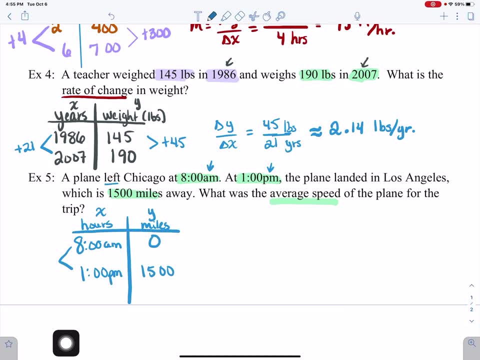 So the change of x? how many hours are in between? It is five hours. How many miles are in between? 1,500.. So to find the rate of change or the average speed, we do the change of x. Sorry.